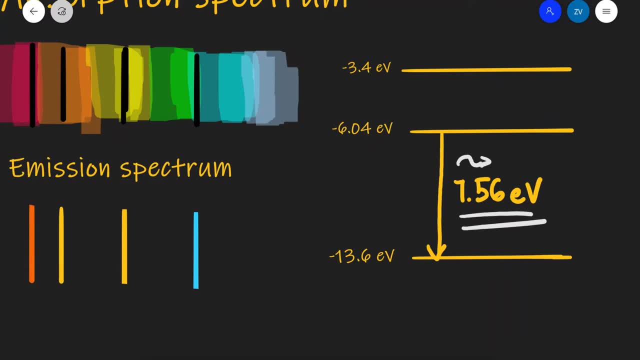 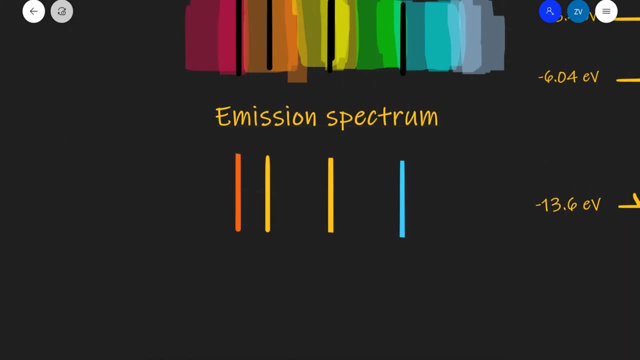 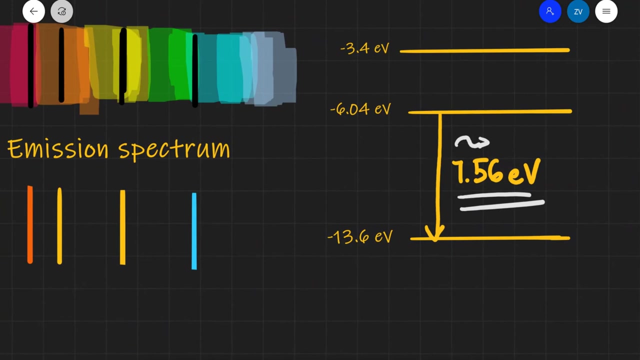 emerging at that precise energy When we heat up a gas, for instance. if we were to heat up hydrogen or a different gas, we would therefore only get certain wavelengths being emitted, because only certain transitions are allowed. For instance, in this case, over here we could have this transition like, so We can also. 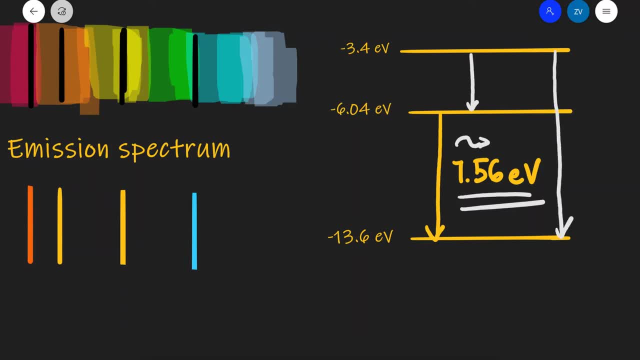 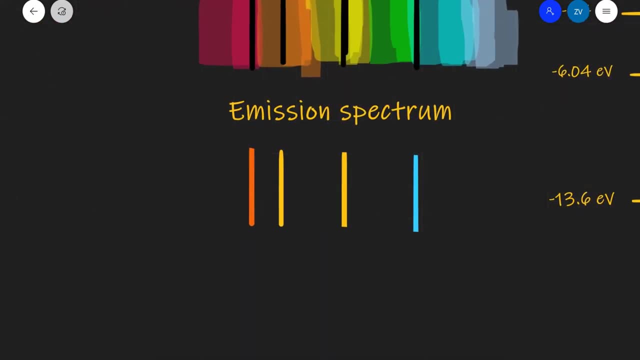 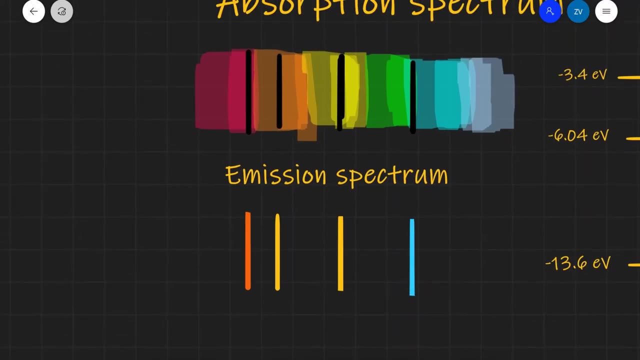 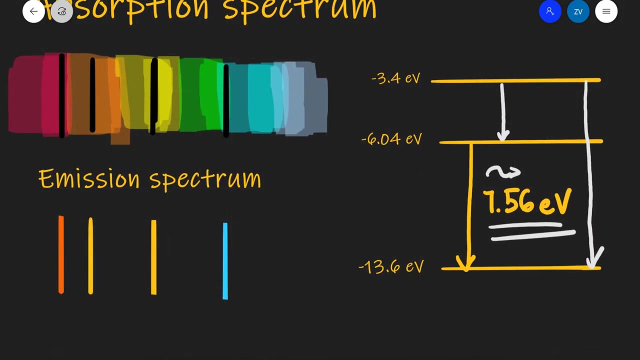 have this transition and only those three are going to be allowed. Every gas has its signature in its emission spectrum. Now the same is absolutely true for absorption. So, for instance, if I had this gas over here with the energy levels shown over here, I 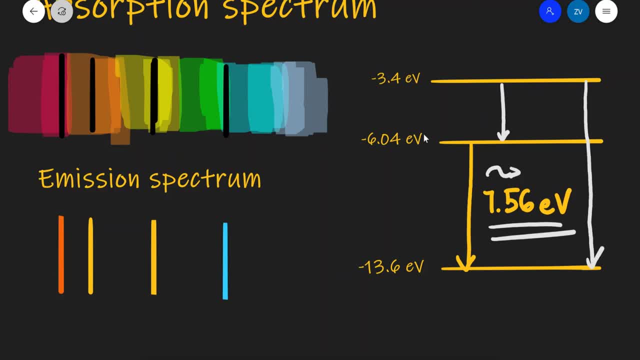 could have exactly the same transitions would be allowed, however in reverse. So in reverse, if an electron is in the ground state, only this transition would be allowed. Then if it's over here, only this transition would be allowed. And if we give it quite a lot. 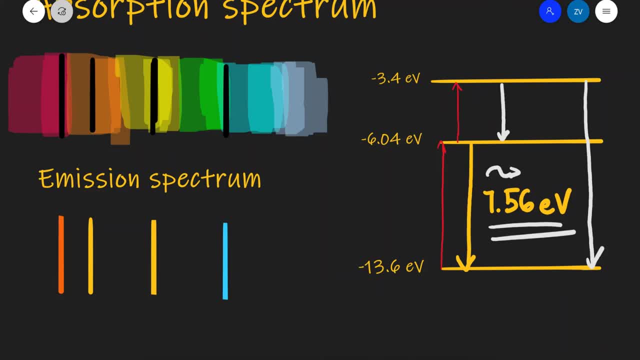 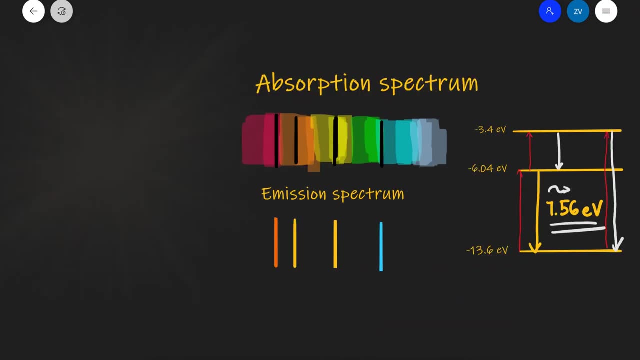 of energy. the transition from the ground state all the way to the third state will also be allowed. Now how is an absorption spectrum really formed in detail? Let's have a look. So let's imagine that we have a star. Now this star is going to be. 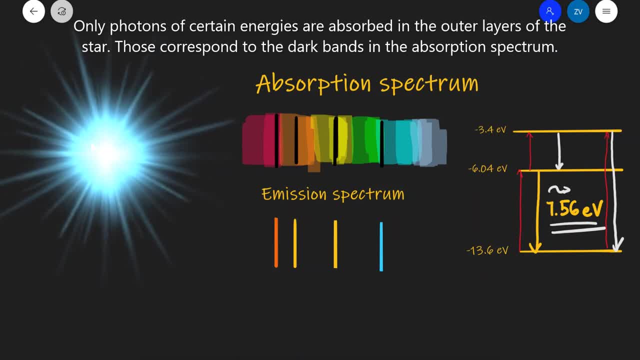 emitting photons across the entire spectrum. However, as the photons propagate, only certain energy of photons are going to be absorbed in the surface of the star and, in general, throughout the outer layers of the star. Now, those specific energies are going to correspond to the specific energies that can be absorbed by whatever